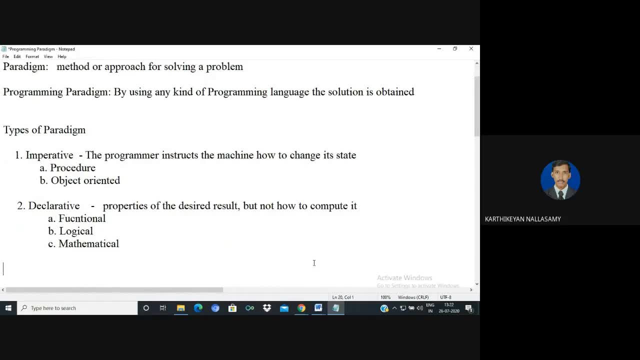 As a programmer or the program will instruct the computer to change its states. It means that the programmer will perform some different kind of calculation by specifying the different kind of functionalities. It means that we are going to write a code and ask the computer to perform that operation based on the instruction given by the programmer. 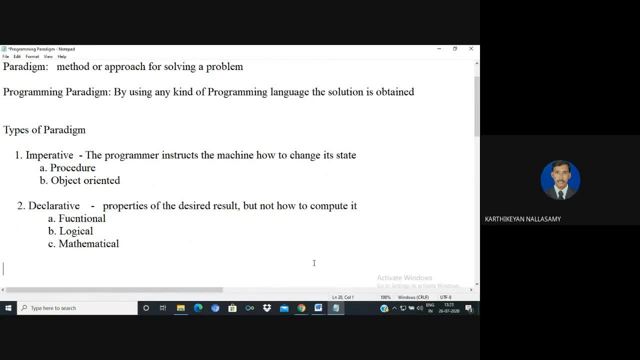 So, the code we have mentioned has to change its states. The change its state means that the values of the values will be changed according to the functionalities which is defined by the programmer. So, the imperative statement and the next one is a declarative. So, normally 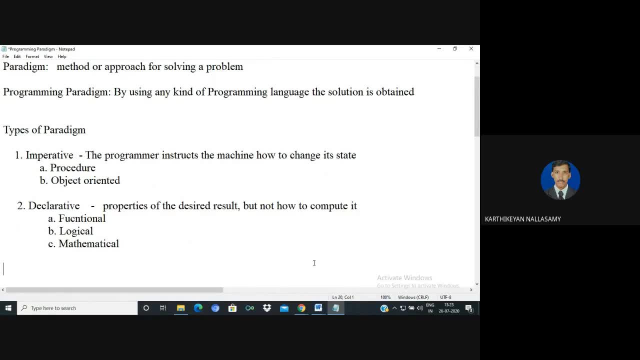 for this declarative method, so we doesn't know how to compute it, but we are going to define the exact output of the results. And so, the machine learning is coming under the concept of declaratives. Okay. So, now come back to the imperative statement. Okay. 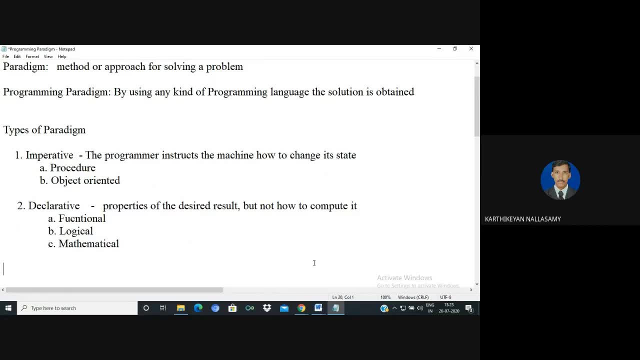 So, in a imperative statement, there are two types of imperative method we are followed. One is procedure-oriented, second one is object-oriented. I will repeat once again. The paradigm is classified into two types. One is imperative paradigm, second one is a declarative paradigm. In an imperative paradigm, we are always, we are instruct the, means we are also define the instruction based on our needs and ask the computer to follow it. So, second one is declarative paradigm. So, in this paradigm, we know what is the output. 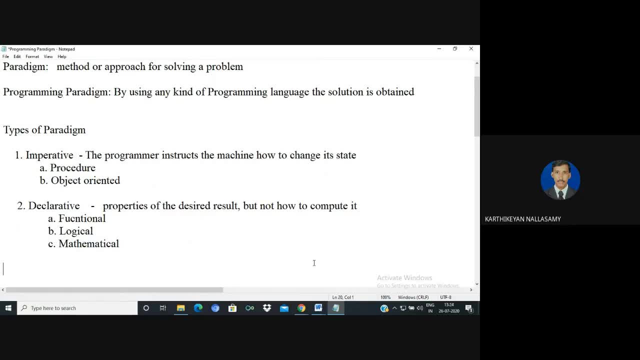 So, we don't know how to exactly compute it. So, based on the functionality or logical or maybe a mathematical, we are defining. So, now we have come to the imperative. Actually, imperative is the majest part of your programming development. So, one is a procedure-oriented programming paradigm. Second one is object-oriented programming paradigm. So, if you are to secure concept of programming, means, procedures-oriented operating paradigm. So, if you are, I mean, if the user, if the user is trying to define Bürger, where is N t? Well, therethe N t. Okay. 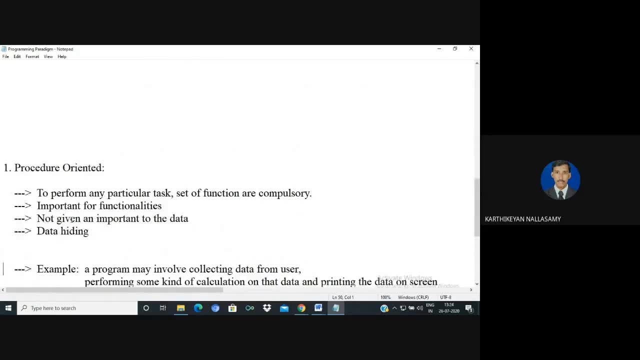 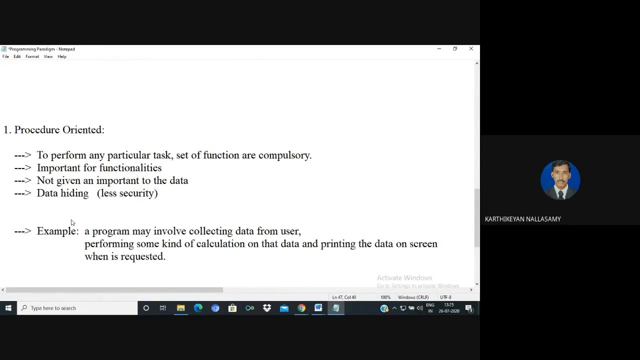 So, I believe that Oui, theren Ji Lady even comes forward there salary there and she is still means if the user looking for one is a particular set task that means that in the procedure oriented paradigm method we are also to looking for the set of functionalities which is associated with it so that means that it is additional functionalities which is identified by the developer and if it is included as a part of the program so and in a procedure orienter we are always given the only importance for functionality rather than the data that means that we are not looking for the values we are always looking for the functionalities and here in procedure oriented no security is possible means only it provides no secret means it's a less security is possible for implementation of informations i will repeat once again uh so in a procedure oriented method so if you are developing any particular kind of a task we are looking means we are once we are developing an application we are looking for some additional functionalities and those additional functionalities must be included in a project even though the customer is not required for a simple example let us take i want to develop one student application for finding the total mark of the three subjects so uh you are the developer as in you are the developer now you are trying to implement the functionality uh so we know that the user 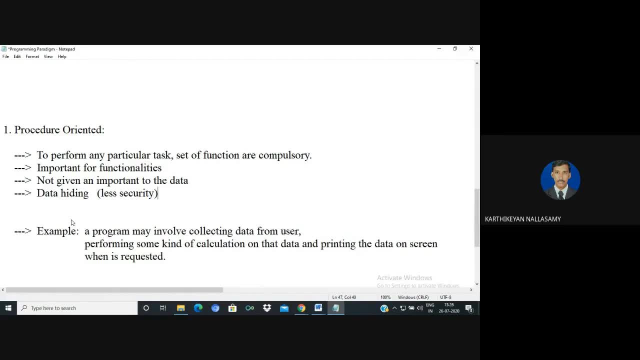 requirement is we want to find the total of the given maps so that is one of the additional is the functionality but as the developer what you need to do was you need to you need to add additional functionalities even though the customer is not expected for example you are trying to calculate the average of the given maps so this is the additional functionality we know that this is a functionality which is associated with our application but the customer is not secure and in the procedure oriented method we are always given a priority for functionalities rather than for the data and again less number of security is there for a data either in the form of global variable or maybe in the form of local variables so uh so uh so here in this procedure oriented method uh so that the cost for the development and the time for the development is high because uh so if you are uh uh for example if you are uh let us uh for example if you are considering one application application development uh so you are looking for some additional functionality also for example assume the particular the task will take 10 minutes to come inside 10 days to complete your projects uh so means complete a project but actually the customer requirements is completed 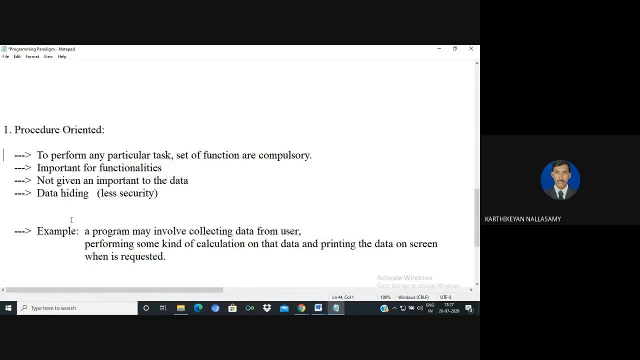 within a day itself uh so uh means the completed within a day itself but if you are looking for some additional functionality for the application you need to consider some additional functionality also functionality even though those additional functionalities is not expected by the customer. So in this situation that means that if you are a customer, I mean you are spending another two more days and try to add those additional functionalities in the project so that we are spending more extra two days for the development and we need to spend some amount of money for the employee to work for those two extra days. 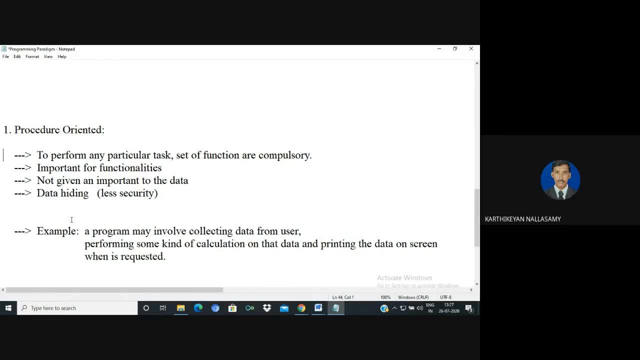 So maybe we can allocate these two members, I mean these two days I mean these members of this project for the summer theme so that the development cost and the project cost may be reduced if you go with only the required functionalities. 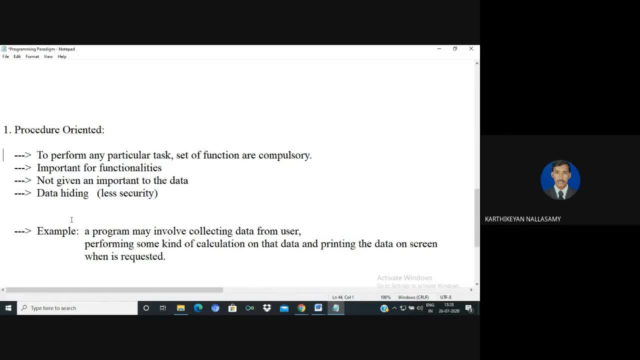 But if you are concentrating on procedure oriented the development cost and the cost for the development, the development cost and the time for the development may be increased because if the user, if the customer is looking for the same additional functionality in the future 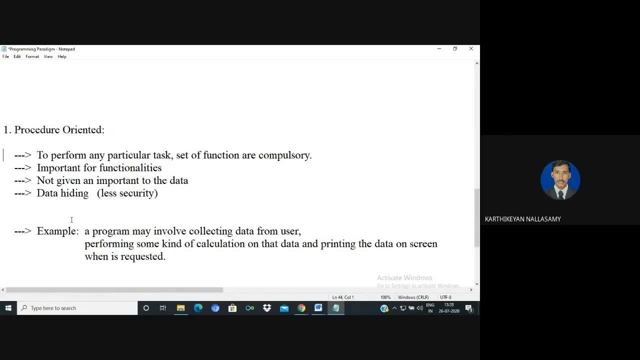 if they are asking a query that these functionalities are missing then simply we can show the SRS and say that this is the requirement is given by you and if that additional functionality you want to add then we can give the request to the customer to give us some extra amount to amount payment for development. 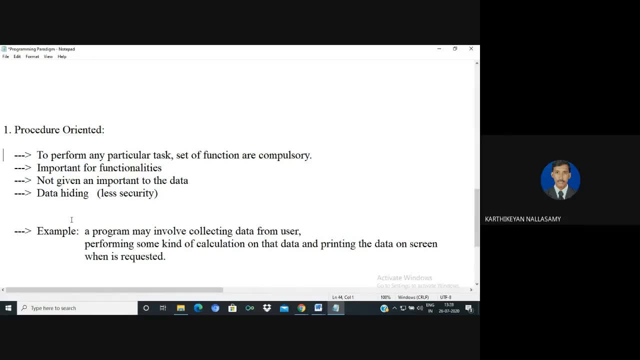 So nowadays the industry is not looking for a procedure oriented they are looking for object oriented method. So in this object oriented method we are looking only for, I mean it's a customer requirements and here they are given a very important for the date and other not rather than for the functionalities. 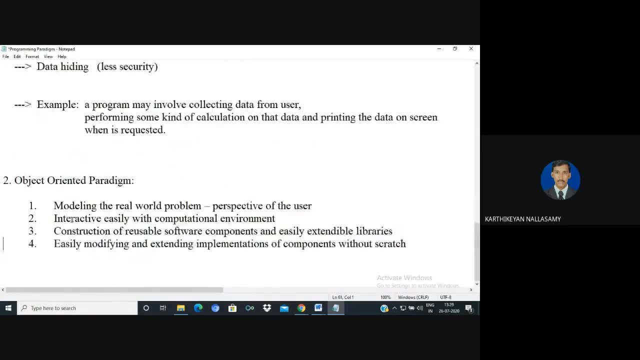 So here this is the major objectives of object oriented programming. So the first one is always we are thinking only for the real world problem. It means that if the what the customer is expected only the those functionalities are implemented in our projects that means that we are not looking for additional functionalities. 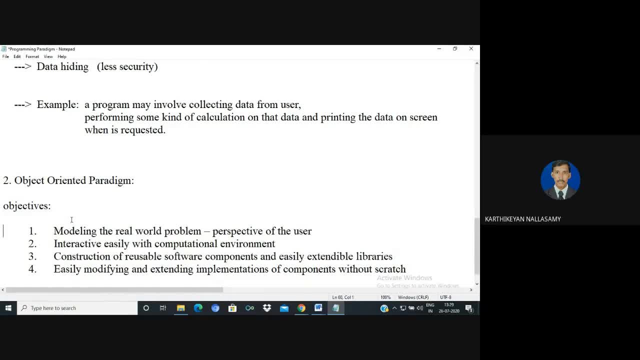 And next one is always we are implementing the with the customer and we are trying to identify the only the major and it's expected requirement. And next one is even though if you are develop this particular application it may be reused for in the future for some other applications. And even easy to, I mean always you are develop by using this object oriented methodology we can easy to modify and extending as a component. 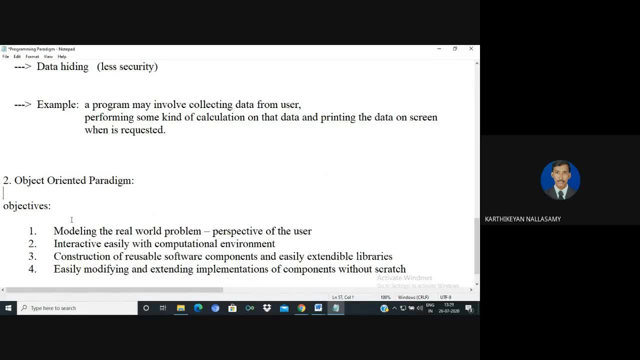 So if you are following the concept of object oriented method 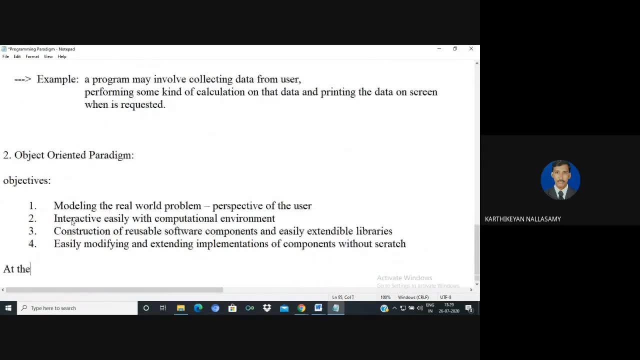 at the end of the project and at the end of the project at the end of the development 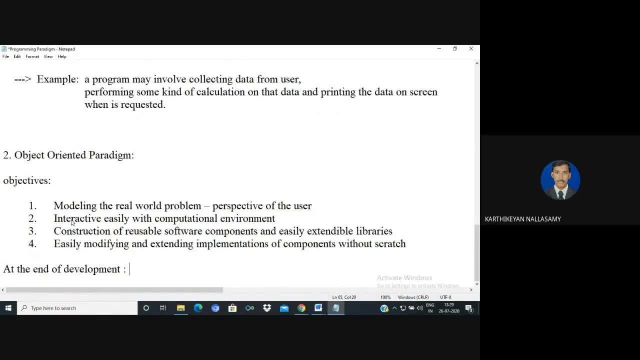 it will be called as component. 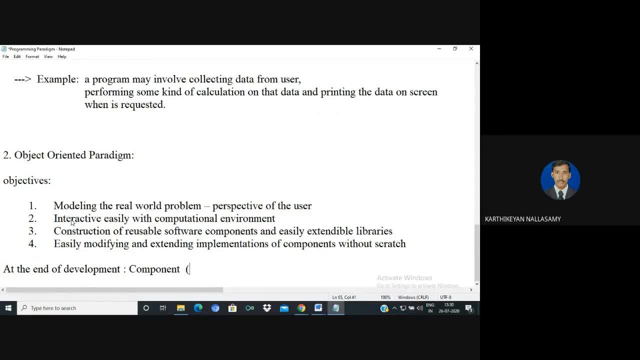 So component is providing all the major task related to the particular 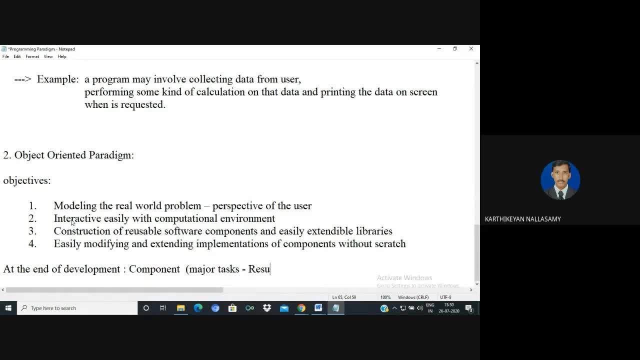 application. If you want it can be reusable. 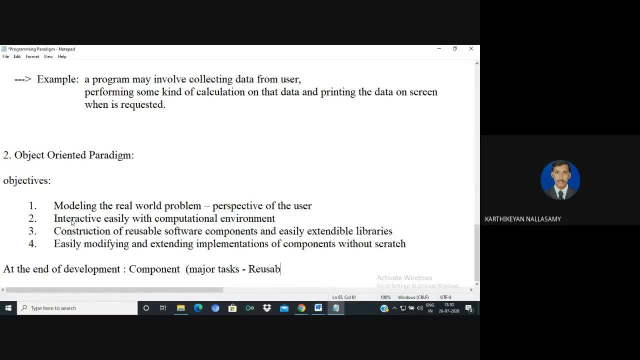 So like that it will be, I mean it will be developed. 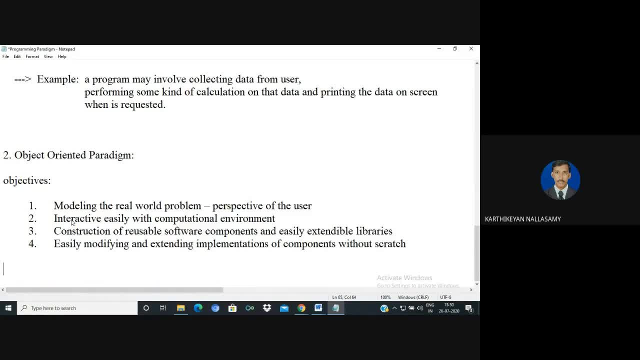 For example we can easy to understand the simple application of object oriented method. 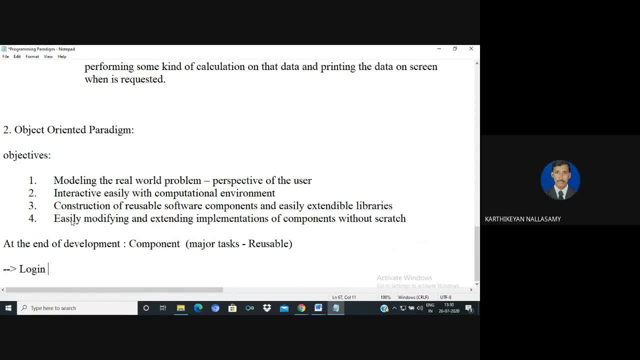 If I am, for example if you want to login into the Google Classroom if you want to login means if you want to join in the Google Classroom 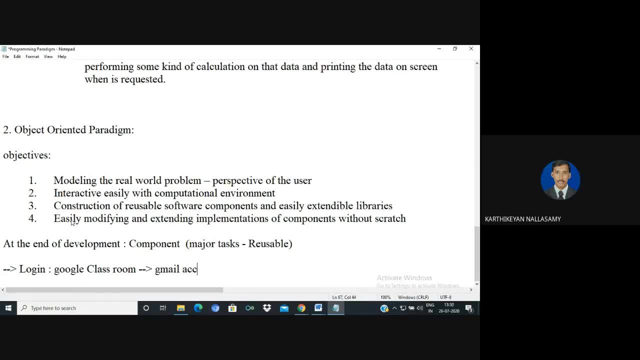 simply just by using Gmail account clear register say next one for example if you want to join in 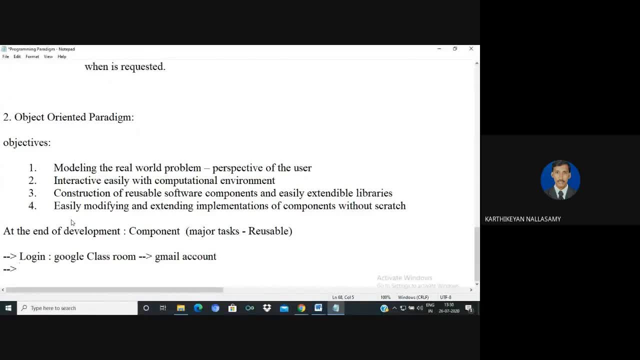 if you want to join in some other applications like if you know that Github sorry IIS Github so by using a Gmail account we can able to link it. It is called reusability. 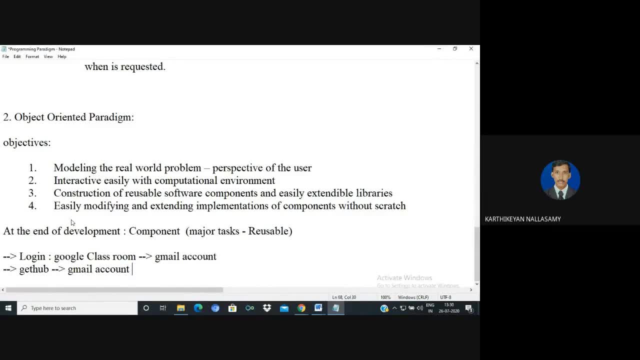 So here as by using a Gmail account simply we are joining in the headhub. 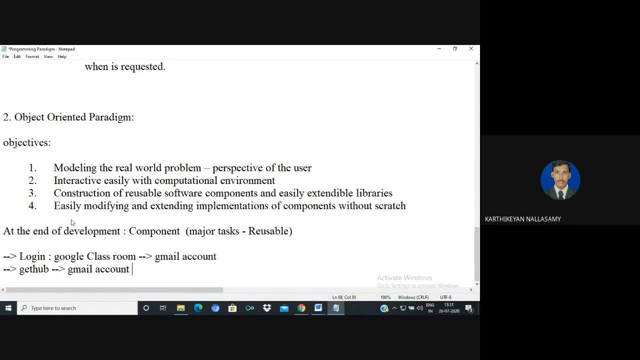 So like that means we called as a Gmail account is a reusable product. 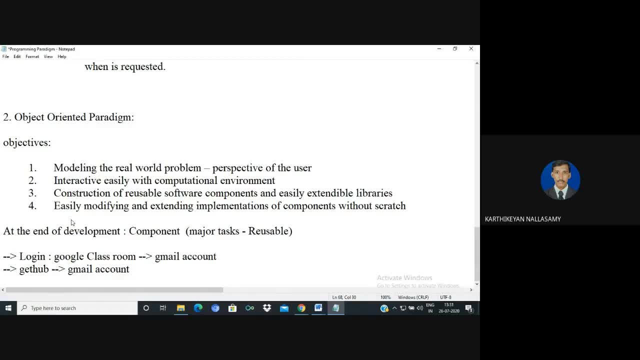 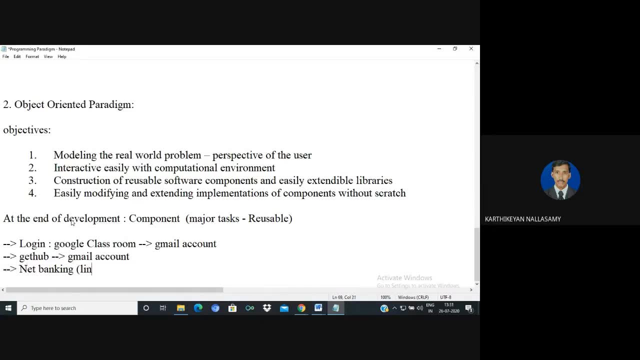 So simply we reused. Same way if you are go with maybe that is called net banking by selecting net banking and just give the linking to the net banking application 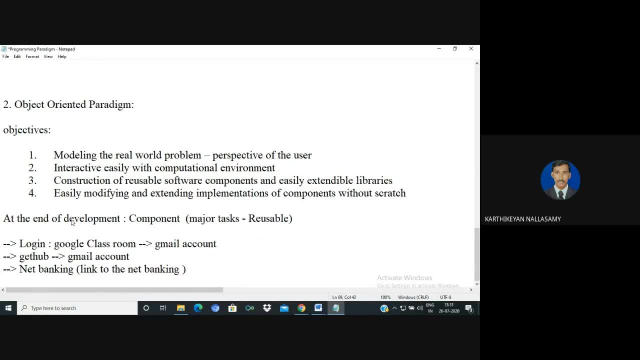 So whenever if you want to transaction automatically the control will be transferred to the corresponding page of that particular bank and it will perform everything and the transaction is performed then again it means that the final 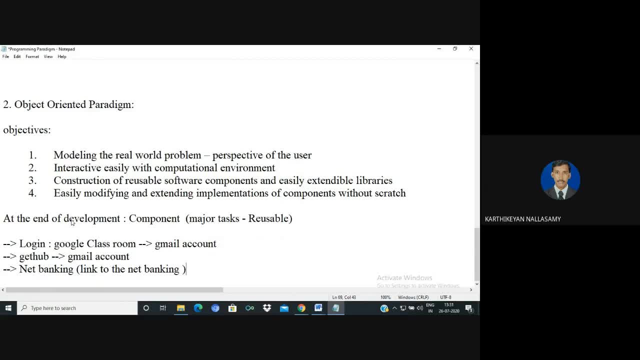 result will be forward to our account and automatically the process by the particular application. 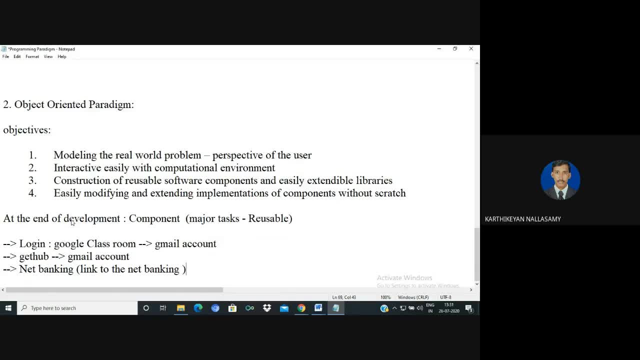 So these are some of the applications which is developed by using object oriented programming. So by using this object oriented because of this object oriented 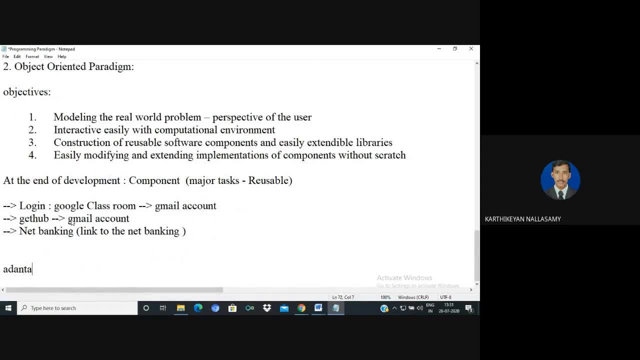 sorry because of this object oriented method just a meter. 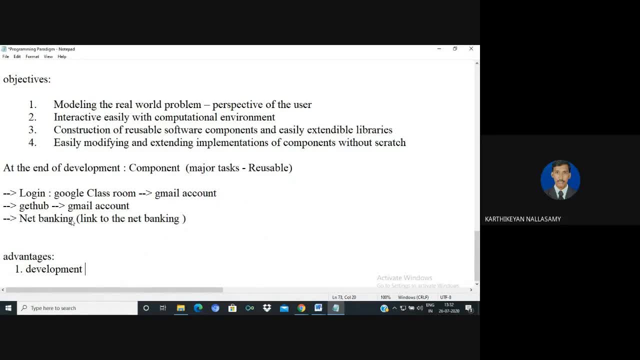 So there are two major major features we have been one is the development cost will be reduced because we are only for modeling the real world problem sorry reduced 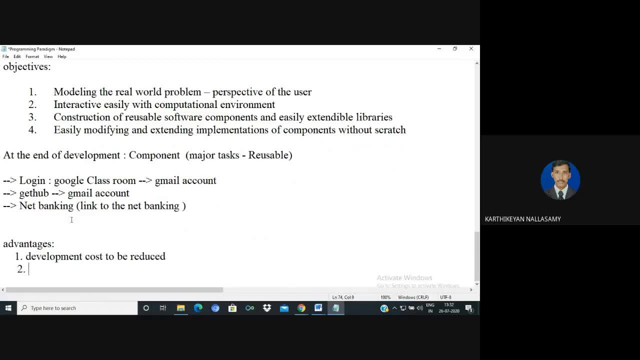 development cost will be reduced and the next one is development time also will be reduced. 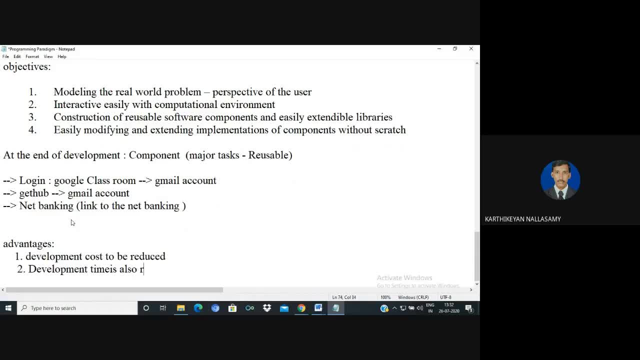 So in the third one is this object oriented methodology provides the concept of reusability. 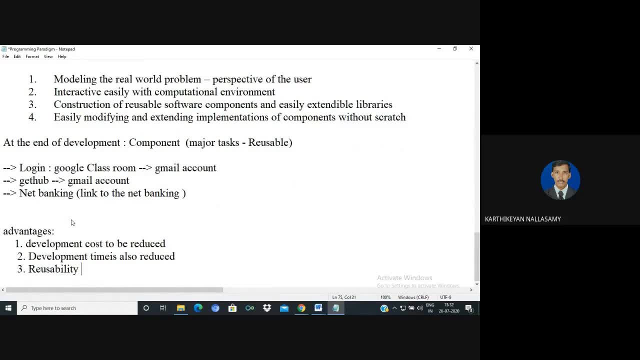 So these are the three major main advantages of means object oriented programming 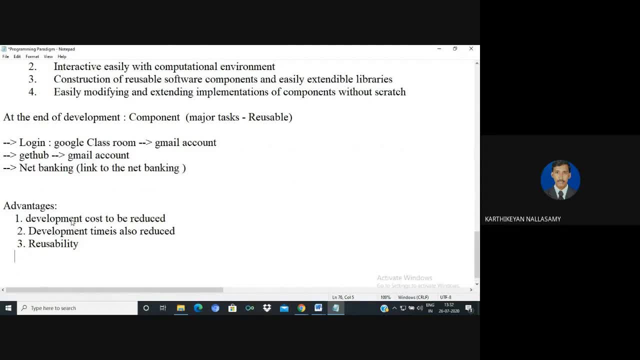 even we have to add in here it provides extra extra security principles by in the form of in the form of access modifiers and next one is the 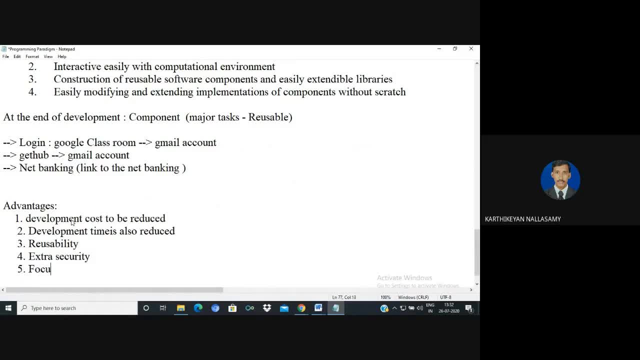 next one is focusing on the data not functions. 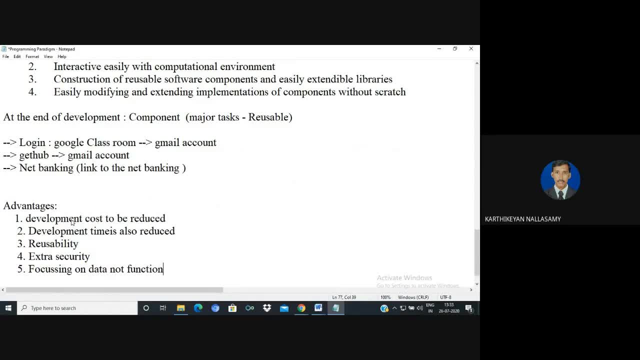 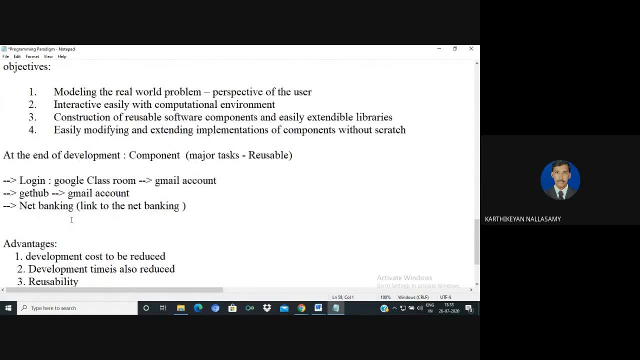 These are some of the advantages of object oriented method and as the all the industry are following means try to follow the concept of object oriented rather than procedure oriented. 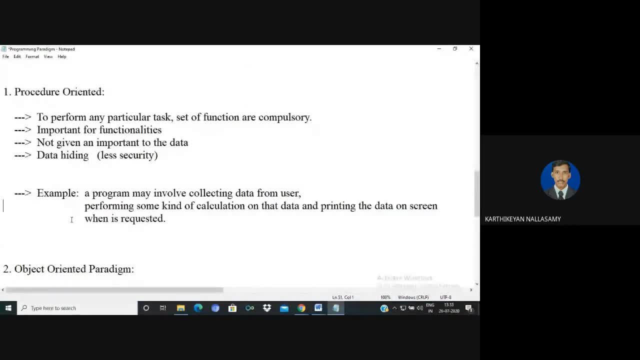 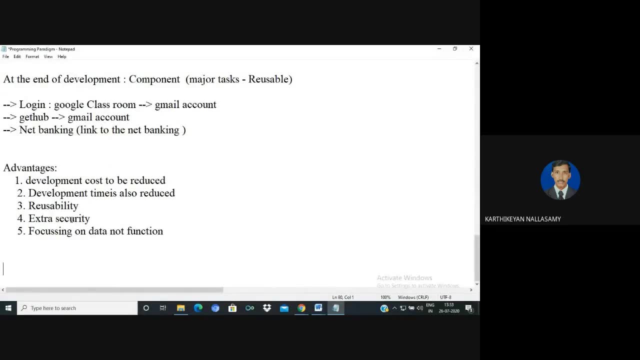 The reason is that we have not developed based on the reusability concept the data hiding is not properly implemented we are implemented in the form of only the local variable as well as global variable but here we are implemented extra security by adding access modifiers. 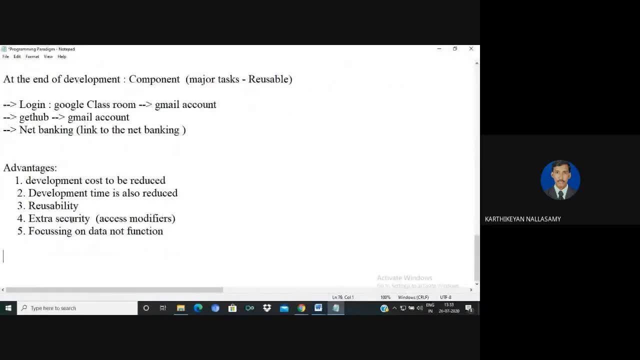 So next one is then the development function in a procedure oriented with an object oriented we mainly focus on data. 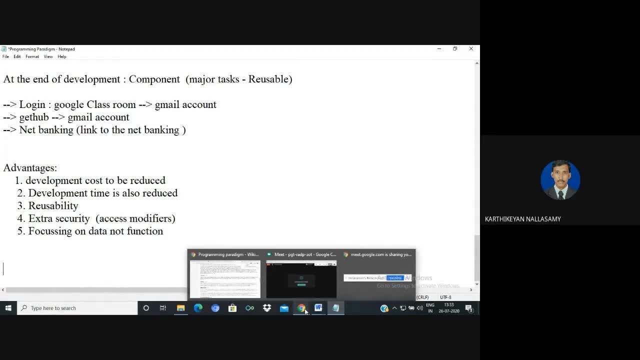 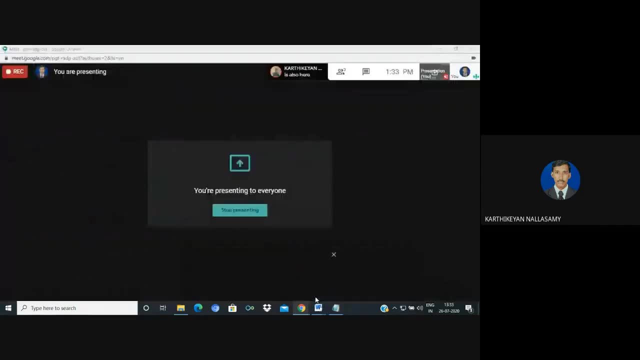 So this is the basic things about object oriented means programming paradigm so from that what we understand that we are always follow object oriented paradigm methodology for the development of any type of application. Thank you.